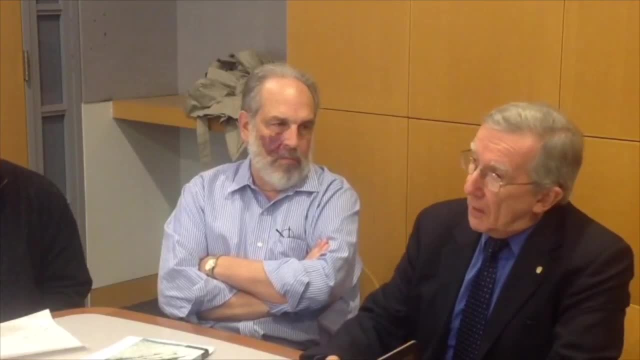 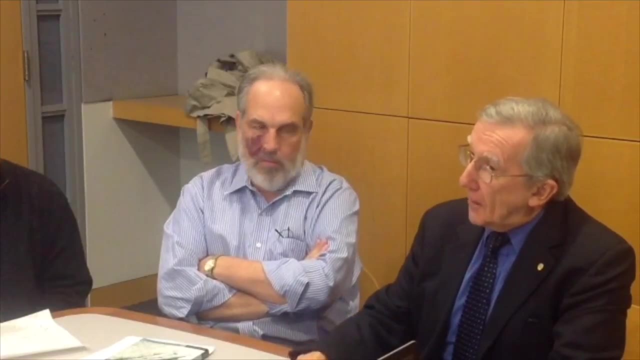 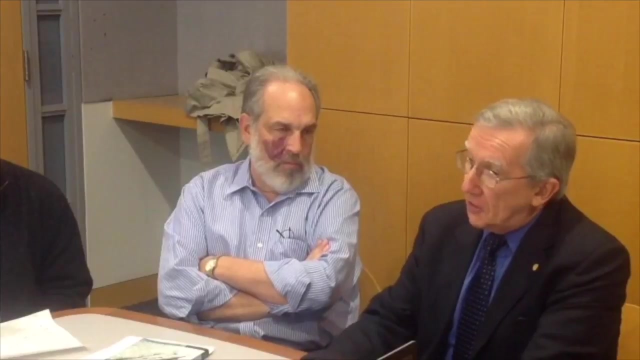 there are plenty of instances where being precautionary means that you look out for subgroups or sub-effects which, in fact, are very unlikely In a world of certainty. one can argue utilitarian ethics applies, That is, if you ban a chemical, you're going to. 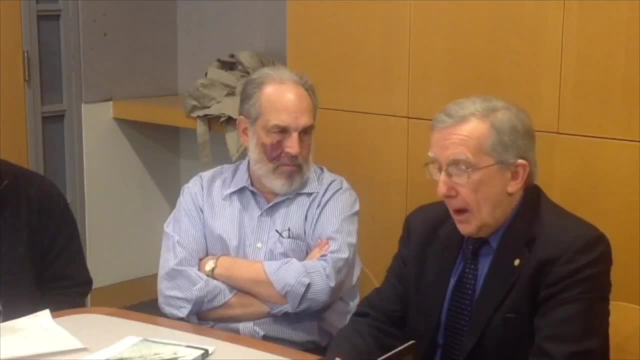 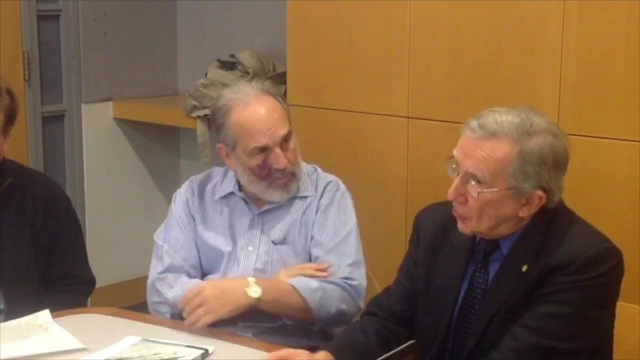 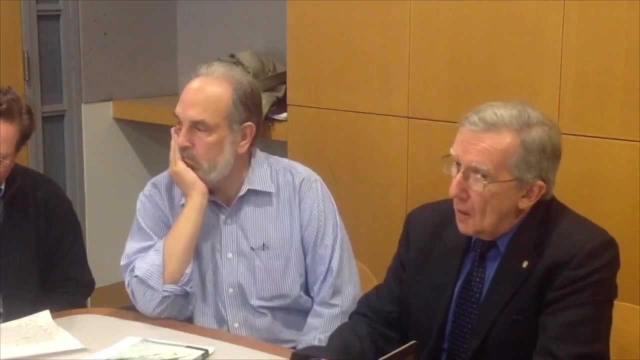 have a certain cost, then you're going to have a certain benefit As soon as the cost becomes uncertain or the benefit becomes uncertain, which is related to risk assessment, because the benefit of controlling a chemical is derived from doing some sort of risk assessment. 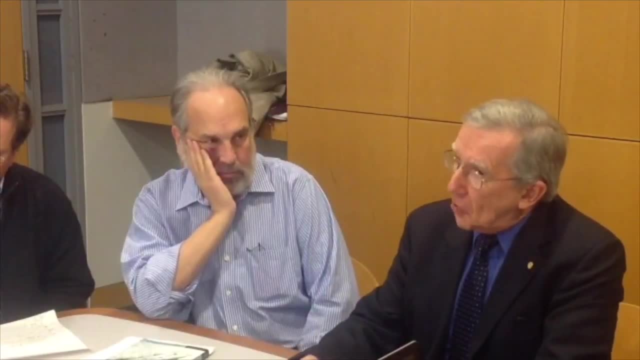 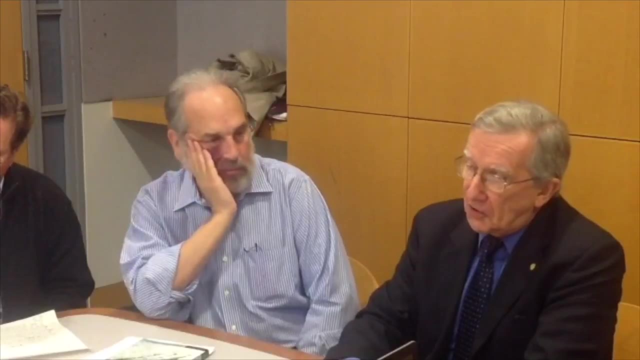 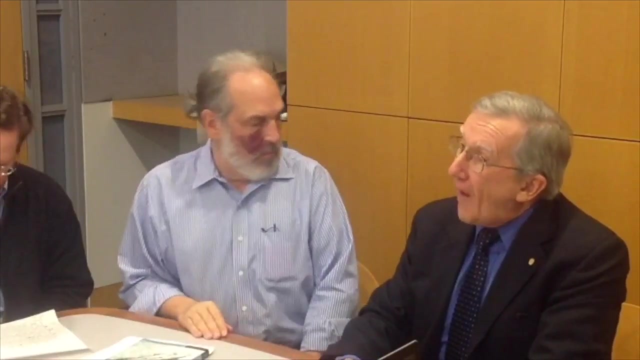 which has high uncertainties in it. But it's not the only thing that has uncertainties: Costs have uncertainties too. So, as soon as you depart from a well-defined benefit and a well-defined cost, utilitarian ethics is no longer important, because what's important is how you value. 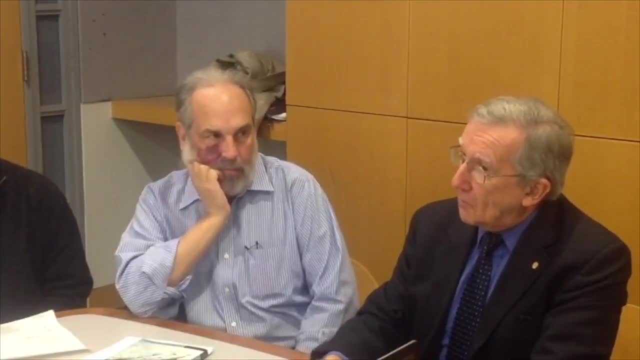 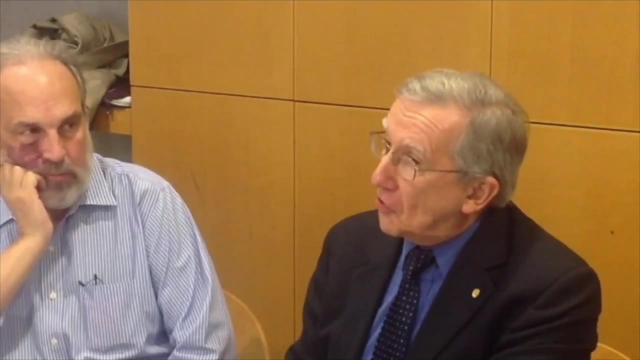 the mistakes that you could make. A Type 1 error comes when you fail to regulate something and it later turns out to be worse than you thought, or at the tails of the distribution of what you think. And a Type 2 error is where you regulate and things turn out to be not. 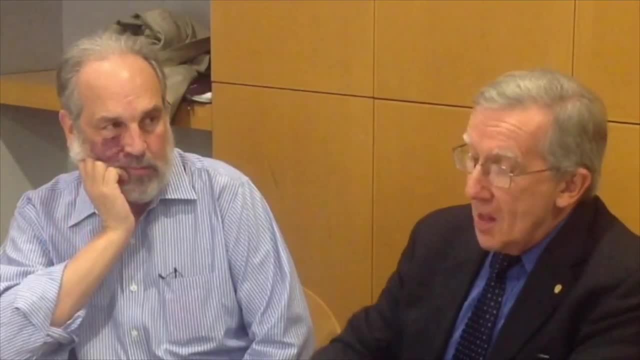 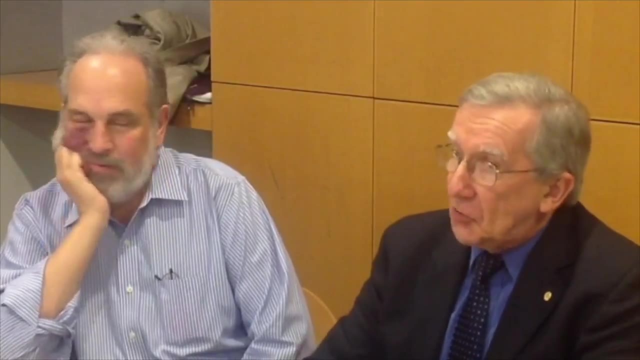 as bad as you thought and impose a higher cost upon. But um, there's a Type 3 error, which is you're working on the wrong problem, And I think that's what you all really missed. The point is that when you ban a chemical, you don't ju-. that isn't. 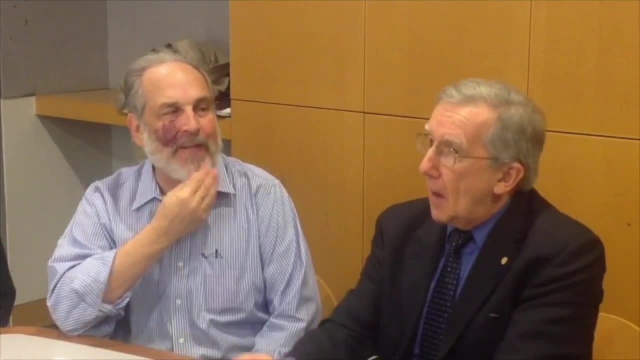 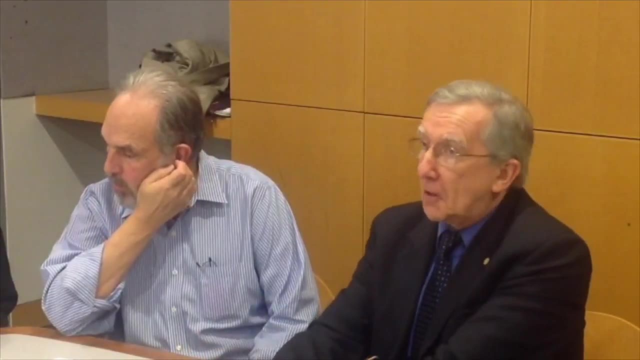 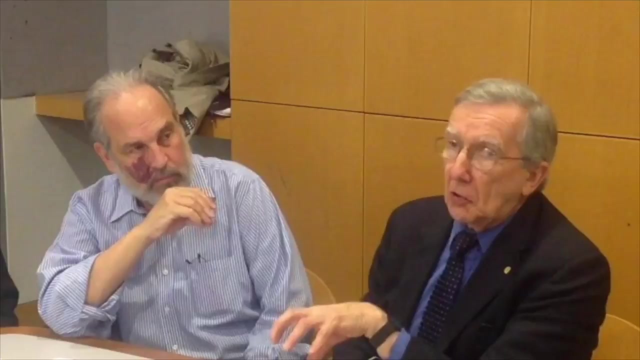 all that happens. What happens is you end up coming face-to-face with a substitute, with an alternative technology, with alternative ways to meet the public needs, And so a straight cost-benefit analysis, even with uncertainty, unless it includes the alternatives, you're. 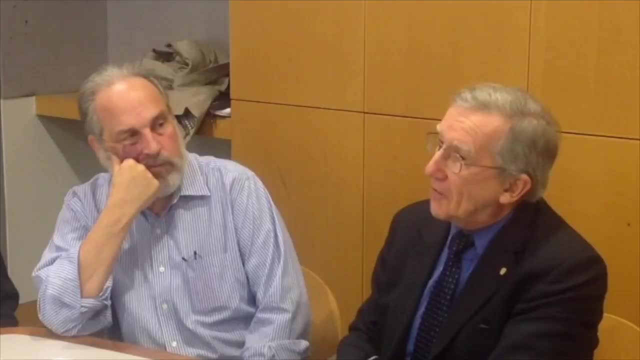 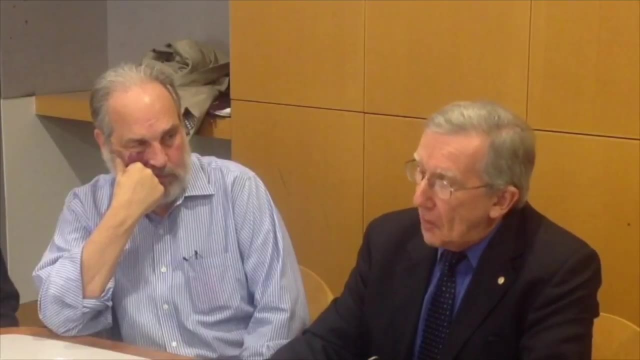 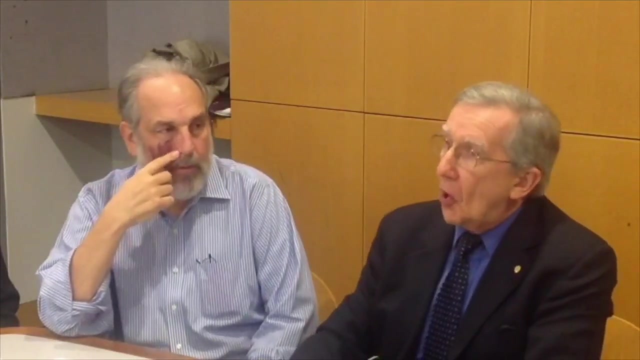 going to end up with a complete analysis, And you can make anything look good, depending upon how you value life or value the environment, And so the precautionary principle properly, which applies when you have great uncertainties, has to ask the question: what are the alternatives? 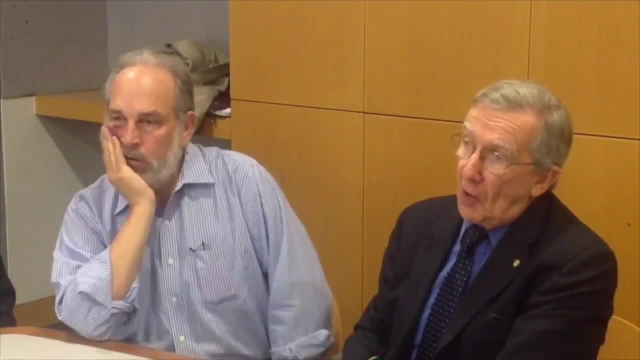 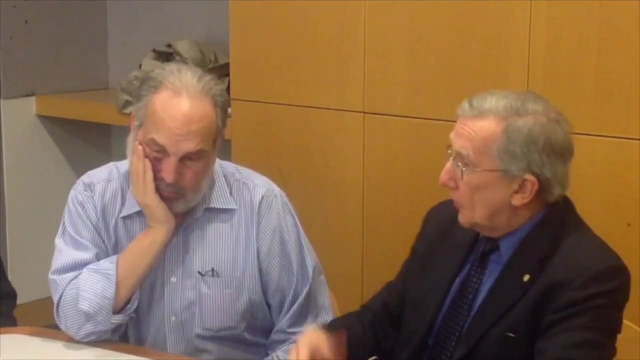 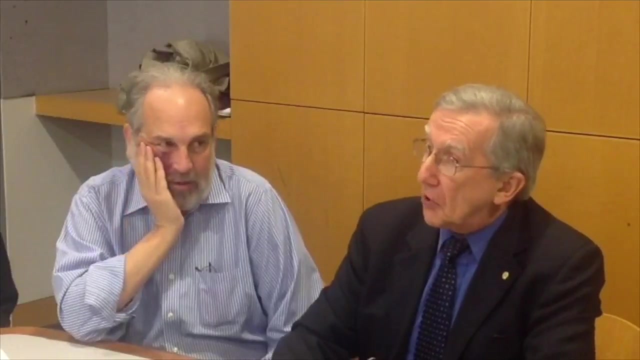 to the action that you've decided to promote, And you know they're alternatives, They're substitutes. I'll give you one more, one more comment on that. I know the work of Cassie Sunstein Well. he and I graduated from the Lane State Law School. I think he is a poor. 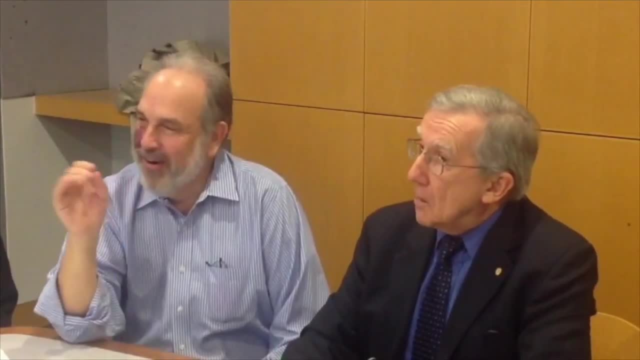 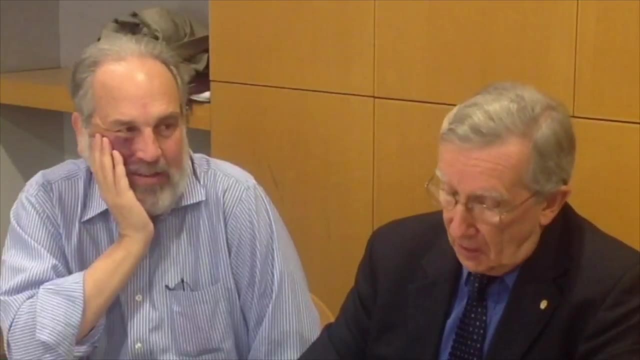 scholar, because I think he does not understand- You heard it here: He does not really understand what, what, what this whole issue is about, Has never, has never really understood it. For example, I mean people say: well, suppose you regulate. 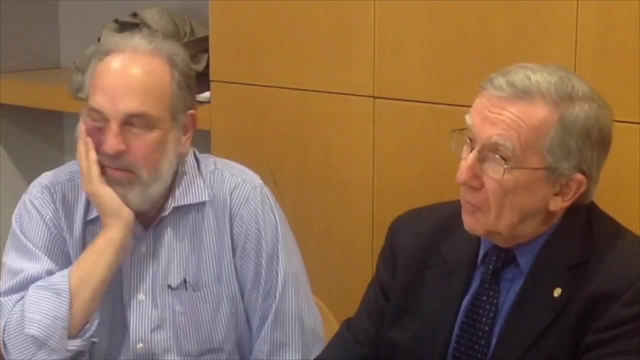 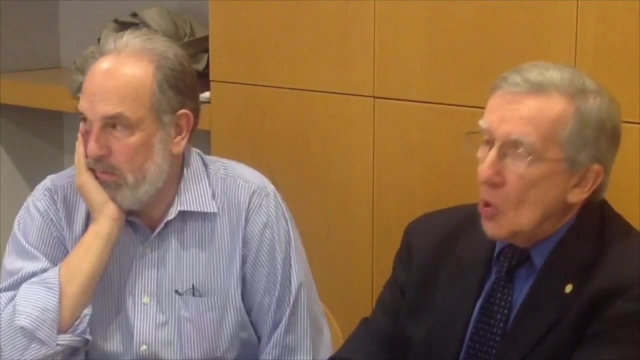 vinyl chloride. You put worker controls on vinyl chloride and the workers now earn a smaller set of dollars. And then you have to go back and say: well, you know, you're not going to pay your salary because the vinyl chloride producer can't afford to pay. 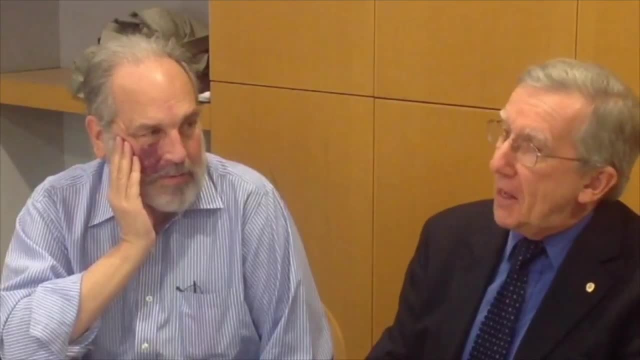 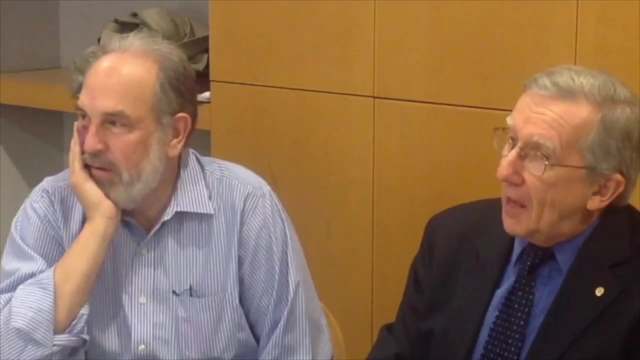 them. So what do they do? They quit their health clubs, They buy less lean hamburger And the health impact- it is argued by by Sunstein- is worse than if you regulated the hazard, because you've made the workers poor and they eat fatty hamburger and don't exercise. 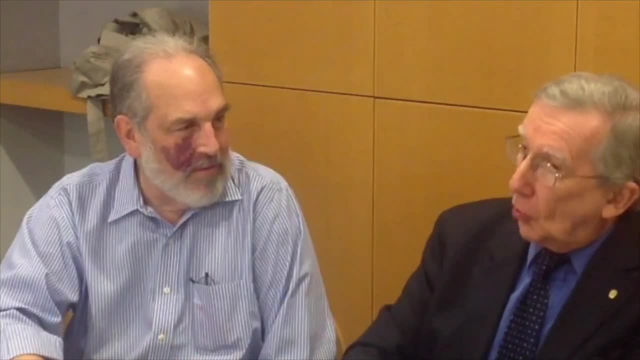 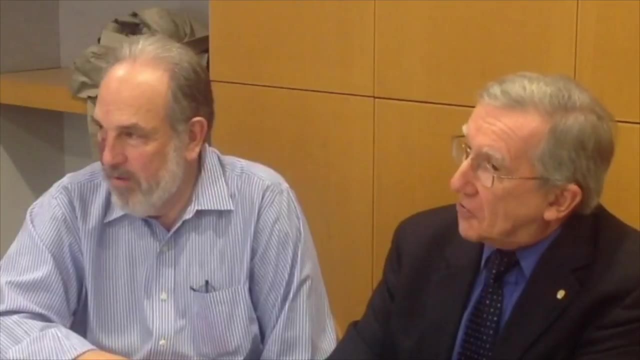 But that doesn't take into account the fact that when you regulate vinyl chloride, what replaces it, let's say, is polyethylene. So those industries increase production, increase the wages of their workers, And then you have to go back and say: well, you know, you're. 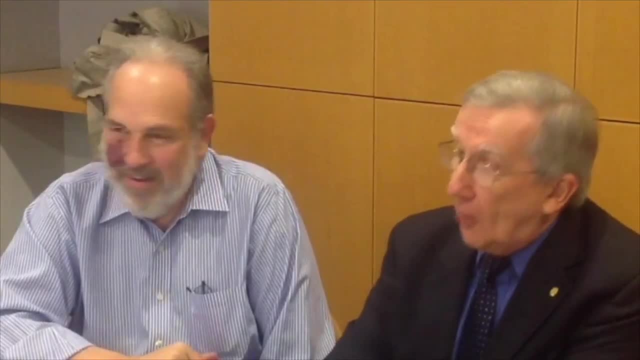 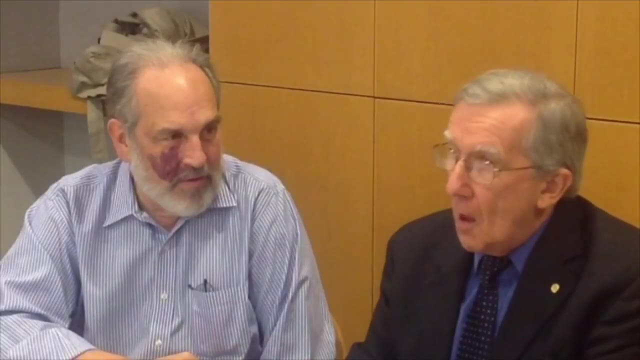 going to fine those workers who now join health clubs and eat lean hamburger. Now, if you're really going to take this calculus to the extreme, you can see how ridiculous it is, because you can't really determine But what you can determine and what regulation has. 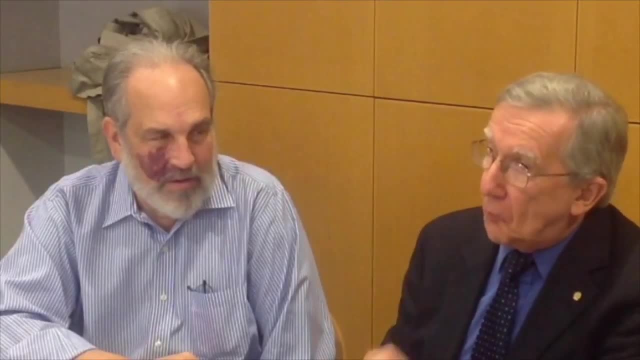 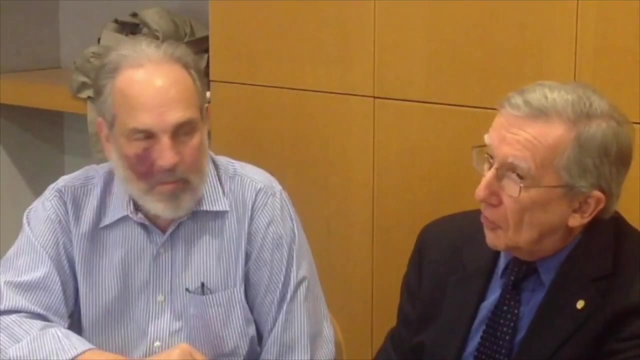 shown is when it's stringent, you don't make marginal changes in production, You make serious shifts in the nature of industrial policy And you shift to non-chemical alternatives. For example, the banning of CFCs didn't just supply one inhalant, which was slightly but better. people started to use pump cans. You sell less product and that's too bad for the producer, but you don't need an inhalant to deliver deodorant or those things, So it is narrowly defined. You work on the wrong problem and you. 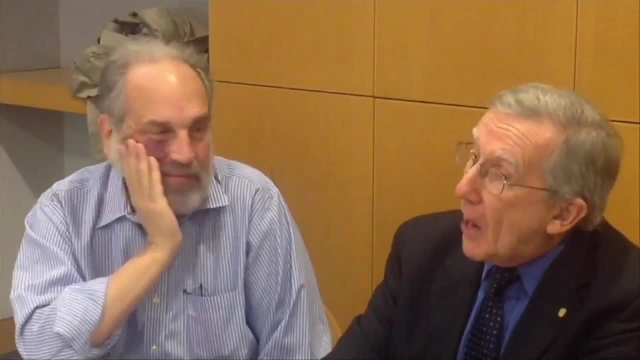 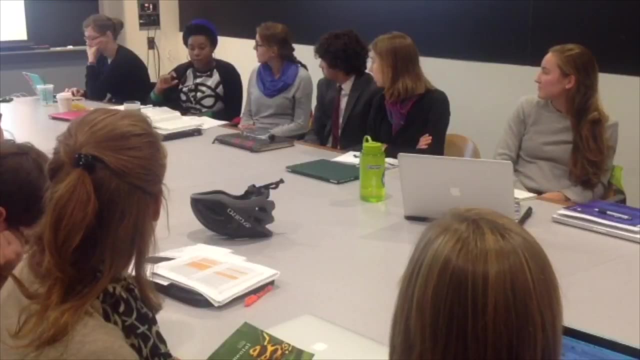 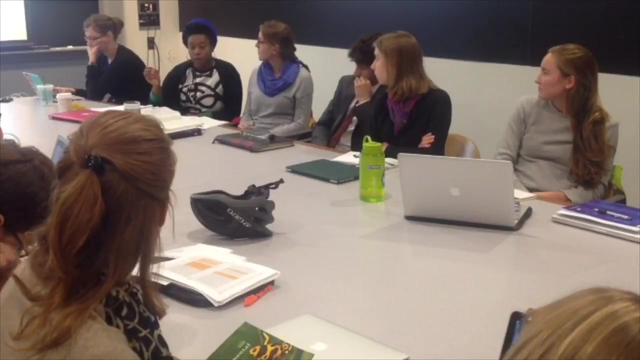 ignore how you feel about air avoidance. That's where the precautionary principle comes in. Go along with it. bring up that point that I think there is a middle ground where, with some things, I think we should look into alternatives and sort of have them as a back seat. 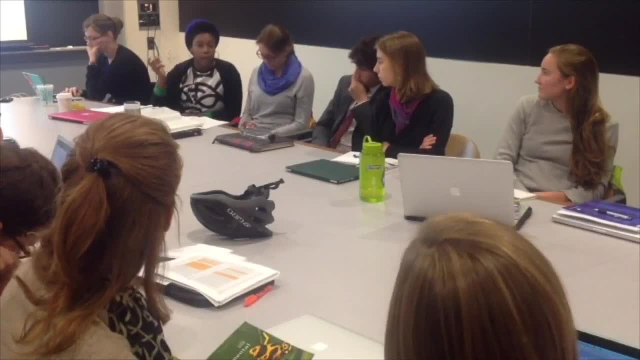 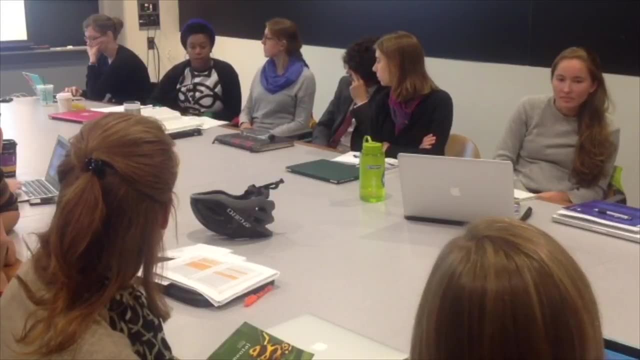 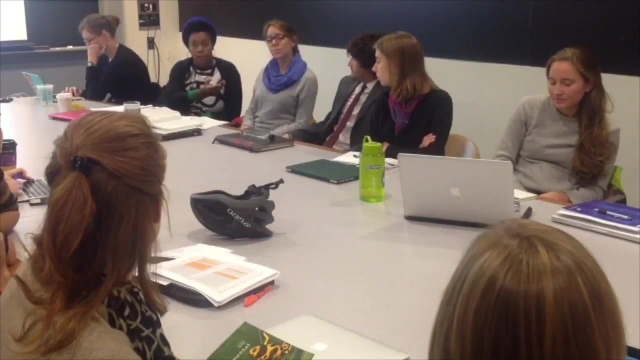 If we find that whatever precautionary action didn't work out, I think it's really dangerous to just ignore other alternatives. Like the Sustain article said, going with that action leads to- Yeah you know- unintended things that maybe could have been a benefit. 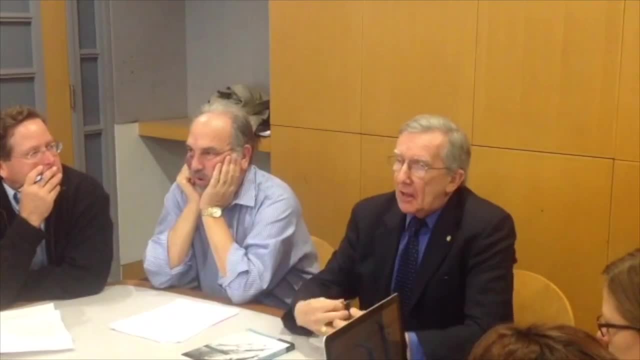 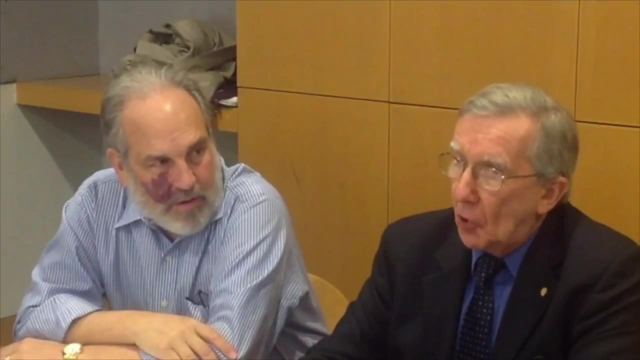 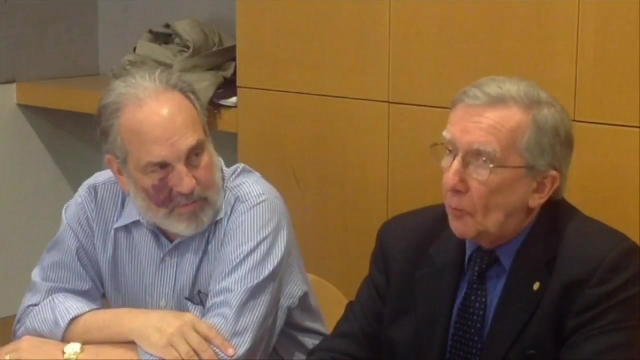 You know, take the global warming situation. You know this middle ground, I think, is a fiction. We either have to regard the probability of serious global impacts as within the realm of possibility, or you don't, And even people who aren't certain about the science. 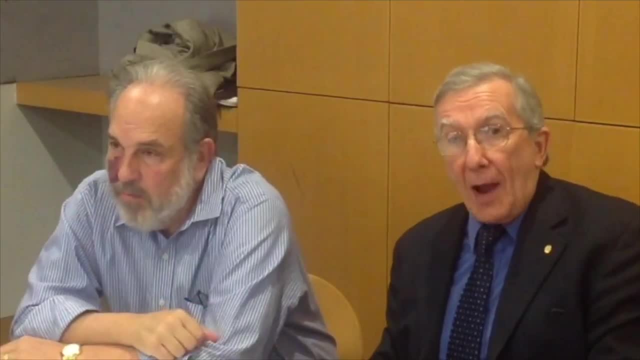 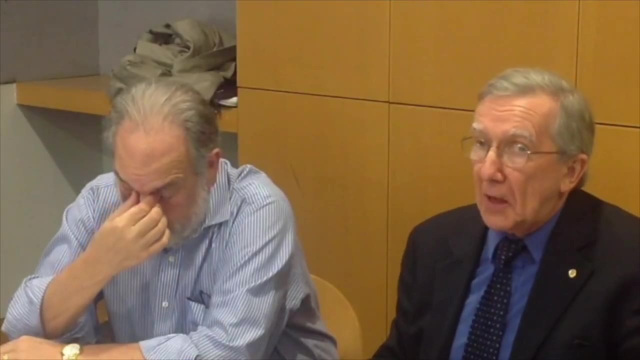 you ask them the question: should we plan for a rising seed level? Should we plan for floods and drafts? Would it be a bad thing to do? And the answer invariably comes: no, it should be a good thing to do, And if you act in a timely fashion, even if you turn out to be wrong, 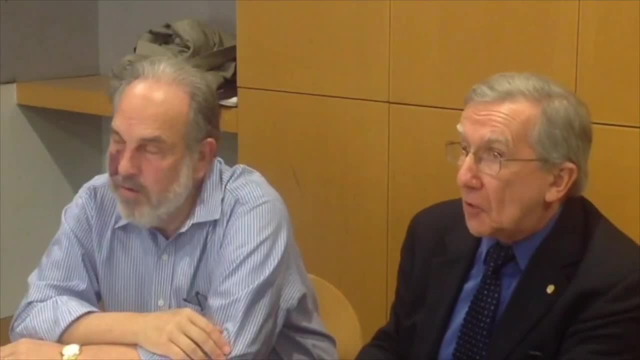 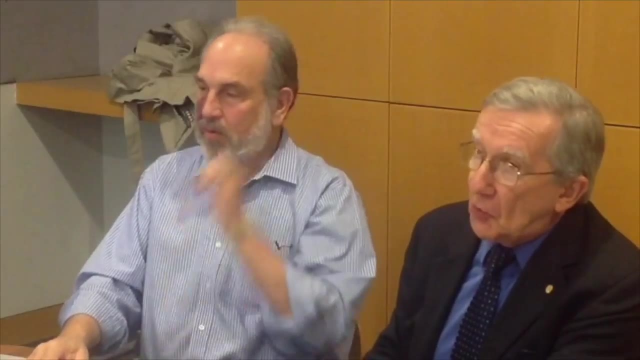 you have imagine what would happen if you turned out to be right. but you turned out to have the coastal cities disappear and Indonesia flinked into the sea. I think the Prashant Principle has been criticized by people who have an economic horse dog in that fight. 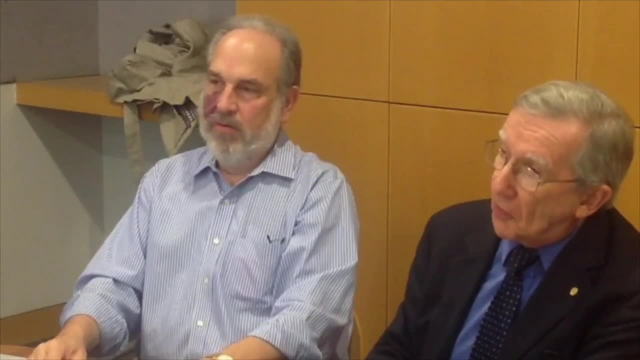 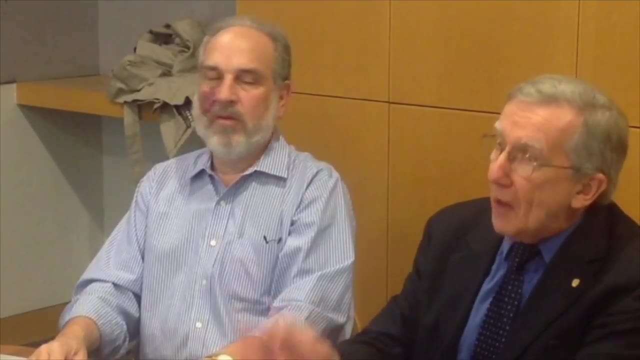 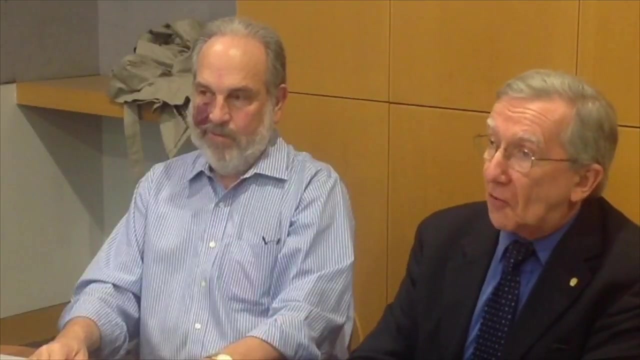 that it's too expensive. It's too expensive and their particular industry will disappear. But the alternative is to have generally other people bear the cost. So who bears the cost and who reads the benefit of the decided policy is very important, And the distributional effects of going one way or the other. 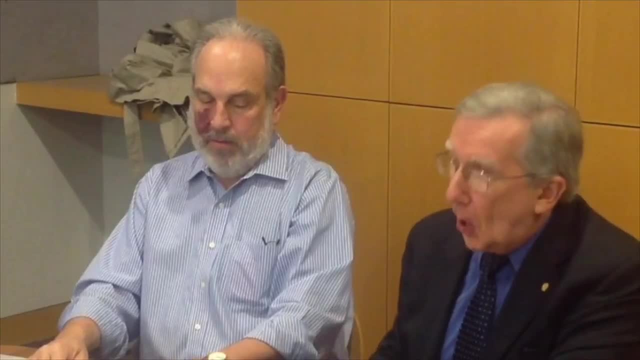 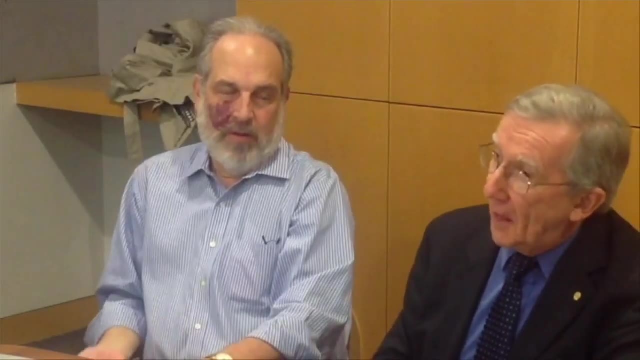 are really serious. I mean, if you decide to put a carbon tax on oil, let me tell you, the petroleum industry will survive. The petroleum industry, If you don't put a carbon tax on it. it's not clean, It's not clear that the plant will survive. 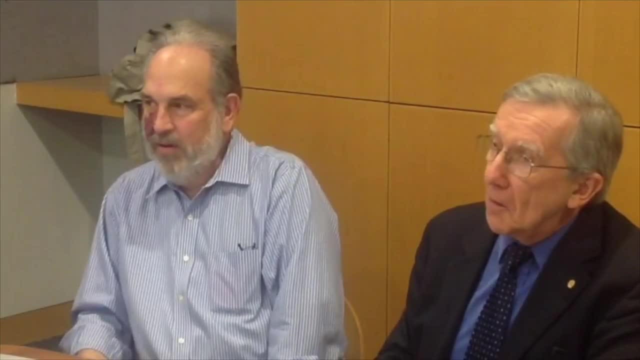 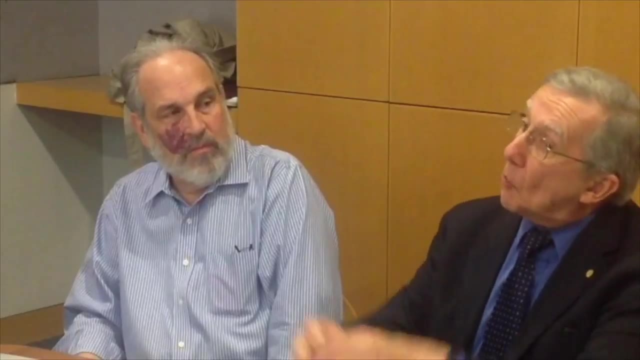 So you have to ask whose ox is being gored. How certain are we that you are producing an irreducible effect on these people And do you want to keep your options open? So I reject the fact that what you're trying to do is find a middle ground. 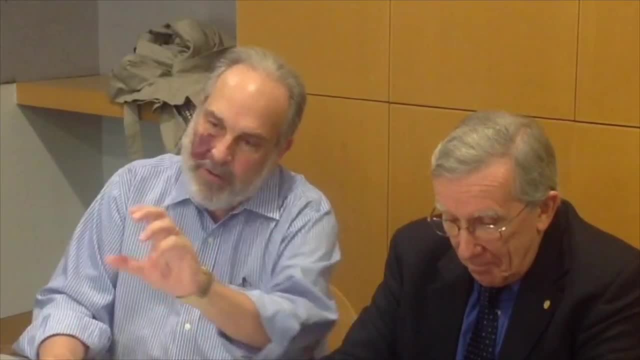 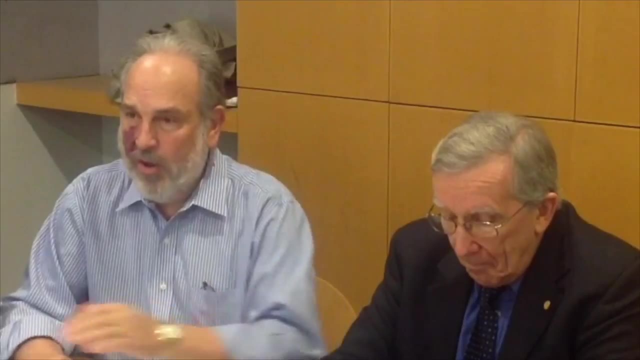 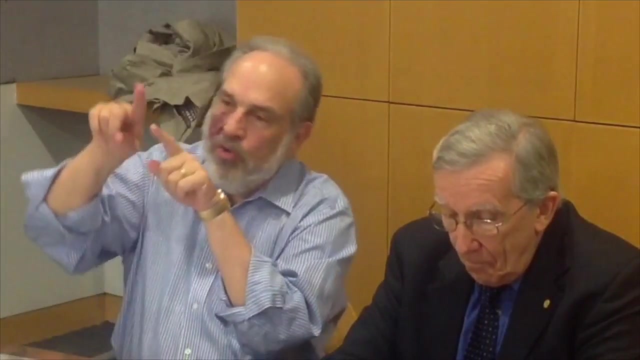 But I want to turn the dial as a last note, one more tick beyond what Nick just said. I believe that- take the climate change example- that if you say let's take this seriously because it might happen that a whole series of second and third order decisions can get made, 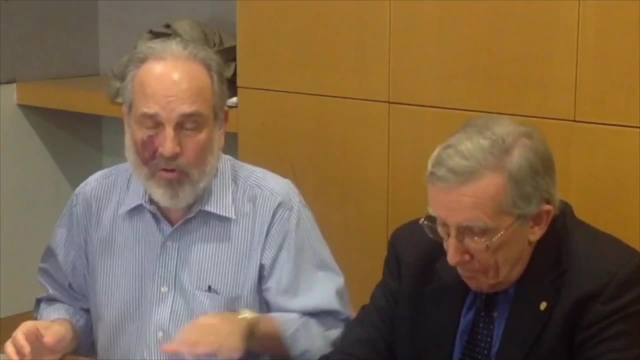 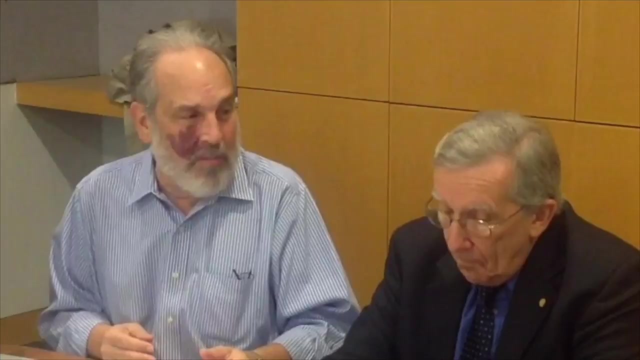 that, in fact, wouldn't get made otherwise. It's related to the point you were making first- And that that will create all kinds of benefits, Because people won't do it to create this benefit. they'll do it to create benefits, But they never would have searched.